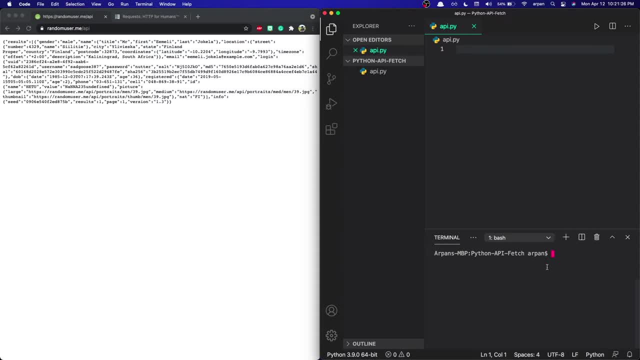 know what request is. request is the library that we're going to use to fetch the API. So open up your terminal and then type in pip3 install requests if you're on Mac, And type in pip install request if you're on Windows. So I'm going to hit enter And, as 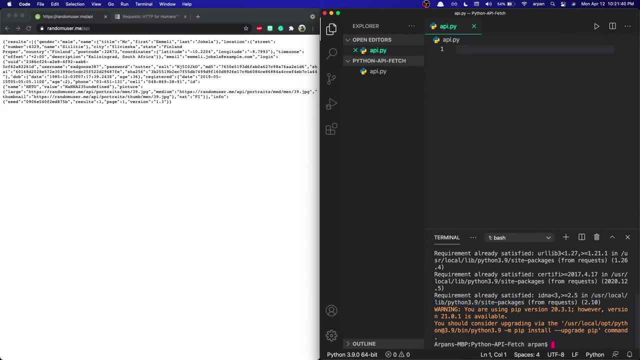 you can see I already have it installed, so it says requirement already satisfied. So I'm just going to clear my terminal for now, And once we've installed it we can import it into our Python file. So we can do import request and this will import the request package. 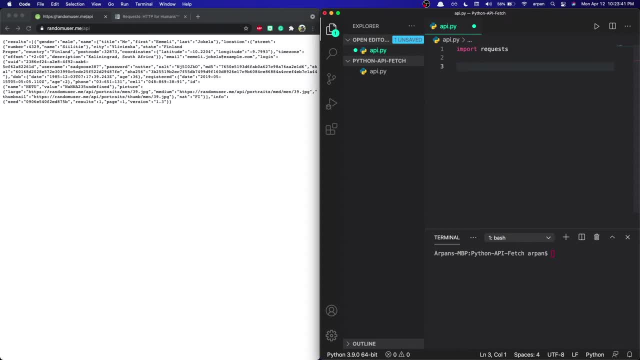 into our app. So next we're going to need a way to connect to this API. So we're going to do: response is equal to requestgethttpspy, And this will connect to the API and will store our response in this response variable, basically. And next we're going to want to know whether our app has connected to it or 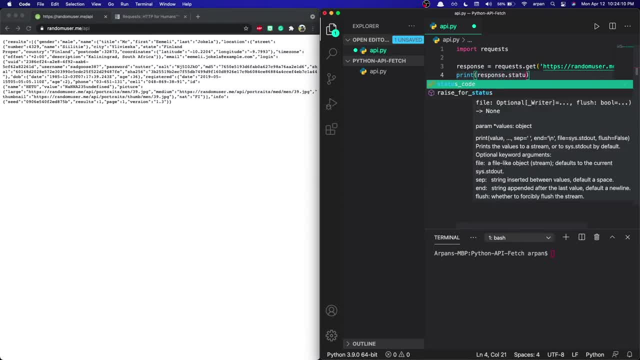 not. so we can just do print responsestatus underscore code And what this will do is basically print out the status code, and the status code will let us know whether our connection was successful or not. If it was successful, it will return 200 out of the status code. 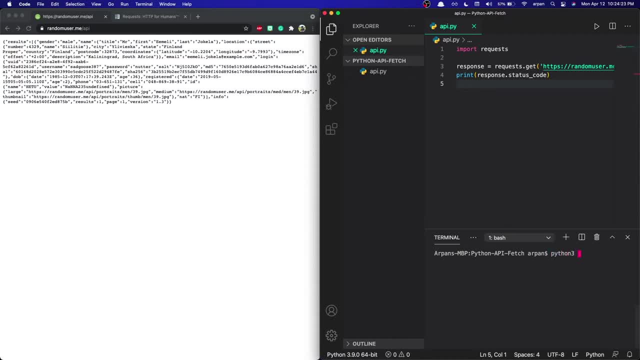 So that's all we need. So that's how we're going to do this. We're going to run our, So we can run this app using python3apipy if you're on Mac and pythonapppy if you're on Windows. So I'm just going to hit enter. 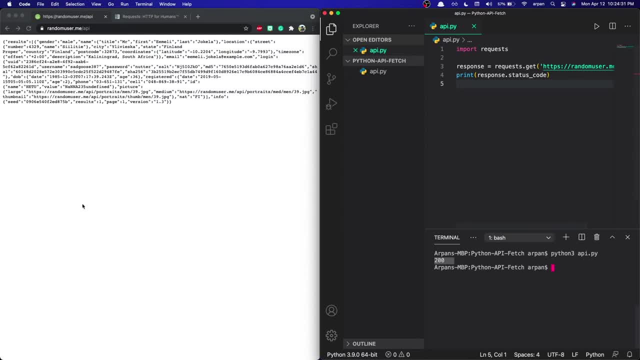 And, as you can see, it returned 200,, meaning that our app is connected successfully to our API. So, since our app has successfully connected to this API, we want to be able to print out the data that we received from the API, And we're going to print that out in JSON. 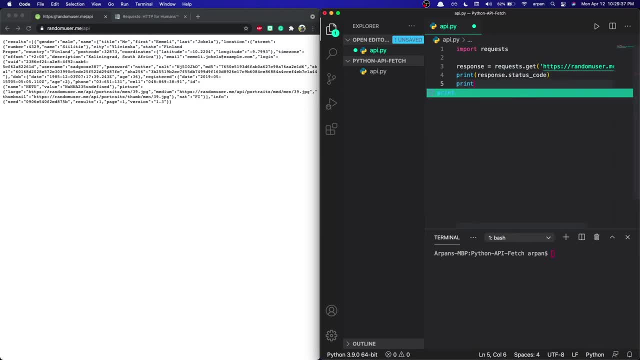 So we can just under this line, we can type in print responsejson, And this will return the JSON data that's returned on this page right here, So we can run our app again. So python3apipy, And then, as you can see, it returned the JSON data as well as the status code for the response. 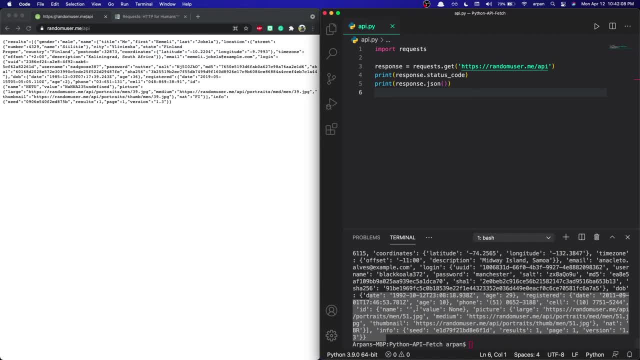 So our API is working, but this data that it's returning looks a bit messy, So what we can do is print out specific parts of the data. So, for example, if we want To print out their gender, we will first need to access this results array. 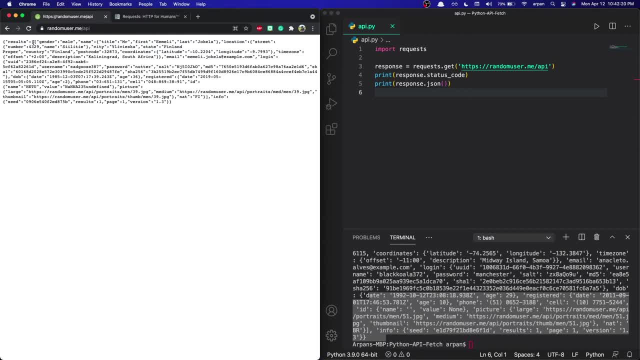 And then, since the gender is located in the first index, we can access the first index, And once we access the first index, we can access the gender. So, in order to print out the gender, I'm just going to create a gender variable and then have this equal to responsejson. 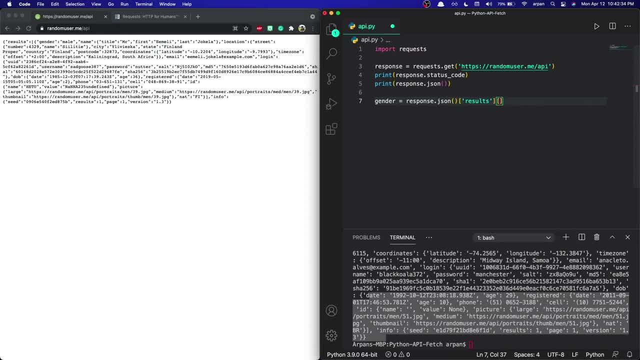 And then we're going to get the results array And then we're going to go into the first index And then, once we're in the first index, we can just access gender, And then next we can just print out gender. So, 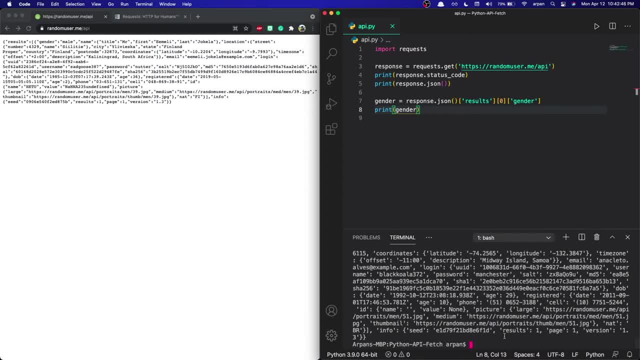 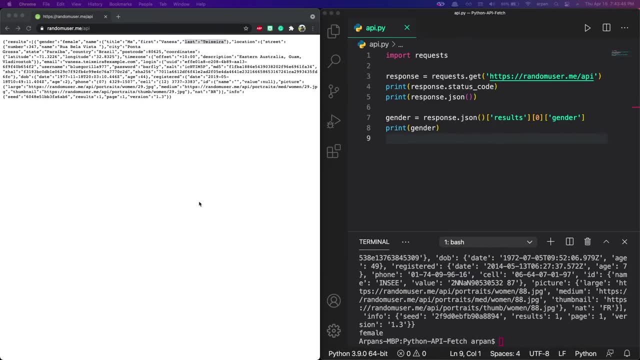 And then save the changes and then rerun the app. So Python 3 APIpy, And as you can see at the bottom, it has successfully returned the gender. All right, So now, since we have their gender, we can basically get anything else. 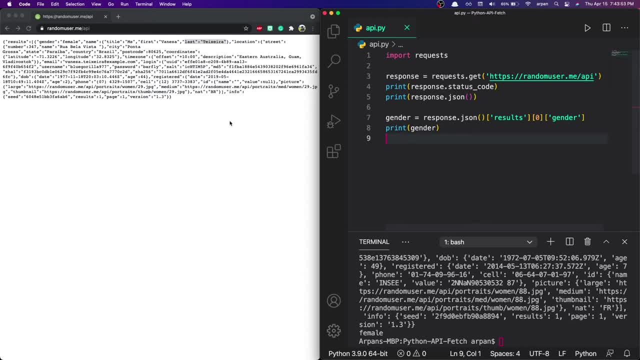 So, for example, let's say that we want to get their first name. In order to get their first name, we're just going to have to access this name right here and then get this first name right there. So in order to do that, I'm just going to create a variable called first underscore name- responsejson. 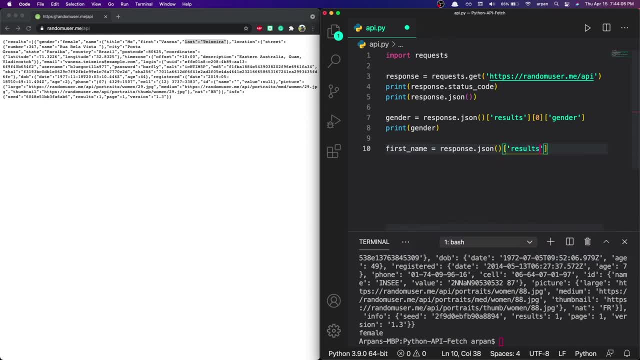 And it's going to be equal to results, and then the first index, and then we're getting the name, and then we're getting the first name And next, all we have to do is just to print first underscore name And then, if we rerun our app, as you can see it printed out the gender and the first name. 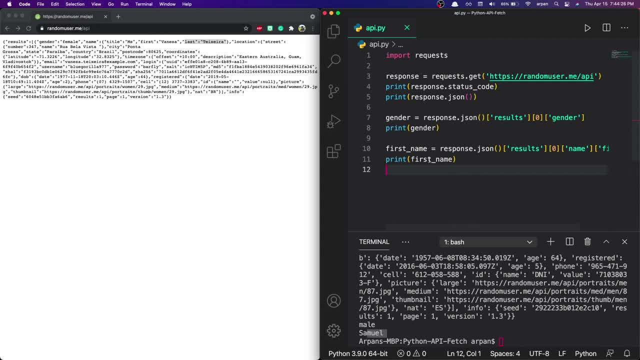 Now, if you want to get the last name, we can do pretty much the same thing, except we're just going to have to pass them last instead of first. So I'm just going to copy these two lines, paste them right below. 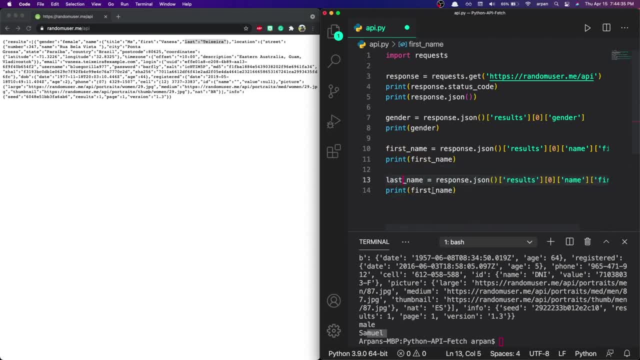 And then I'm just going to rename them, Rename my variable to last name And print last name, And then, also at the end, I'm just going to put last instead of first, And then if we rerun our app, as you can see it printed out the gender, first name and last name. 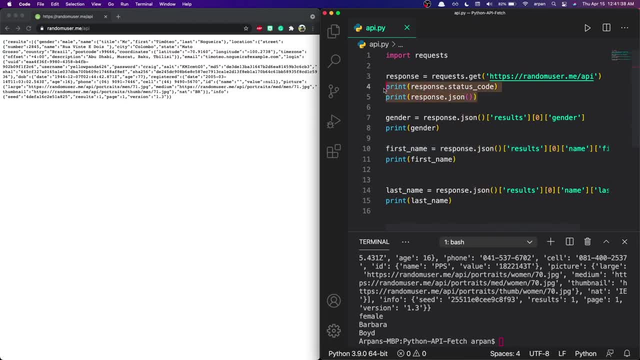 Now, since our code is basically working, we won't be needing this, since these two lines were just for testing purposes, to make sure that our app was connecting to the API. So I'm just going to remove these two lines And, instead of printing out the first and last name separately, we can print it out together. 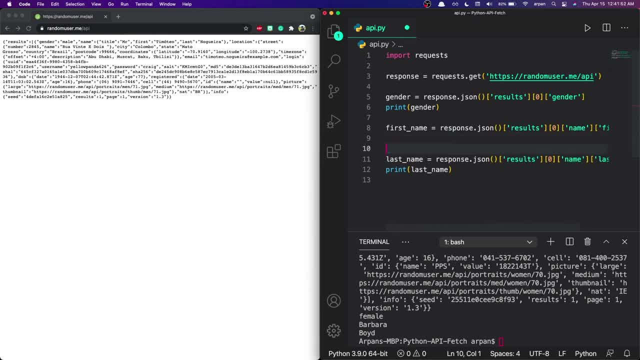 So to do that, I'm just going to remove this first name line And then what we can do is delete that print statement and just type in print then an F string, first name and last name. So last name, right there.